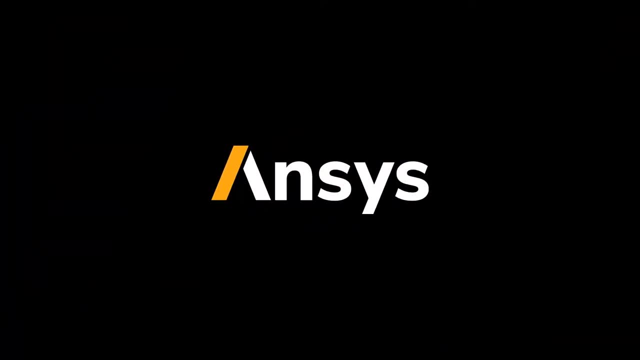 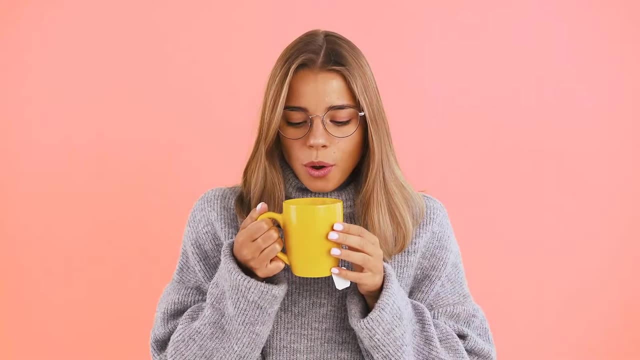 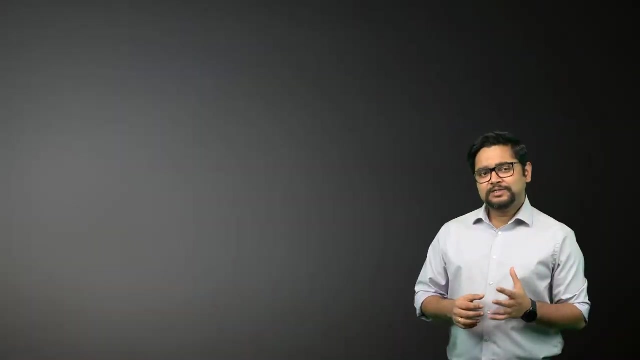 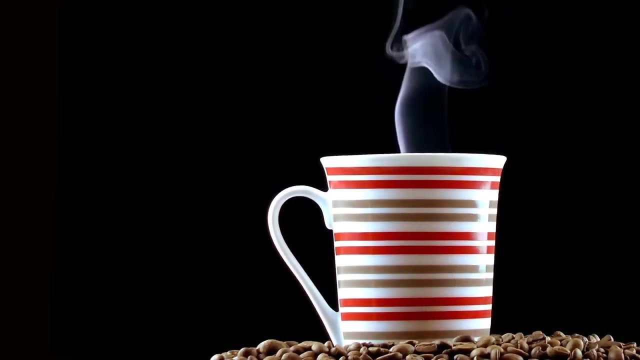 When you blow over a cup of hot coffee to cool it down, you are applying external forcing condition to induce the flow of cool air over the hot fluid. This is known as forced convection. But even if you don't blow over the cup and let it sit on the table, it will slowly but 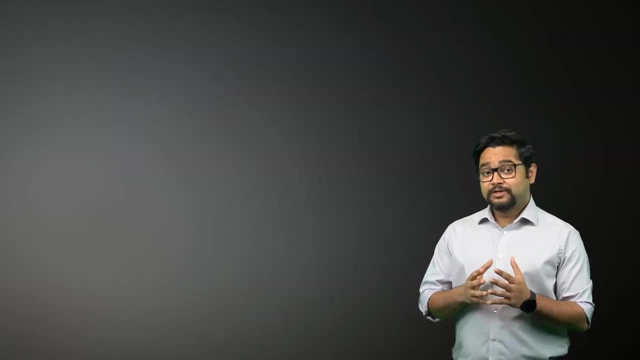 surely cool down. In such situations, where there is no external forcing condition, convection heat transfer still occurs due to the convection currents that exist within the ambient air owing to the density gradients. This is referred to as natural convection and is the focus. 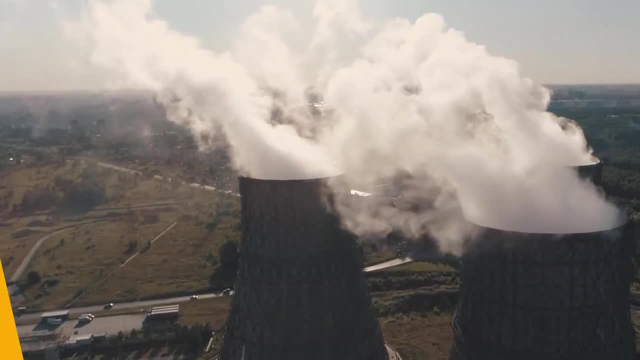 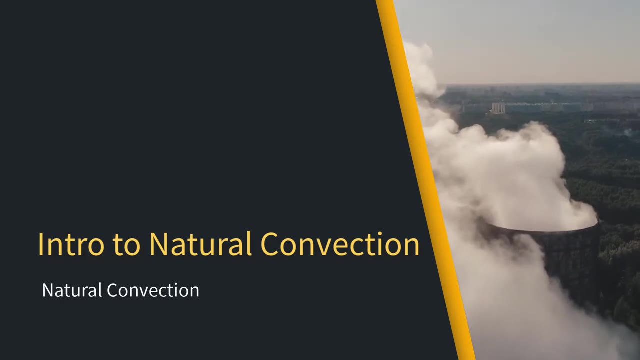 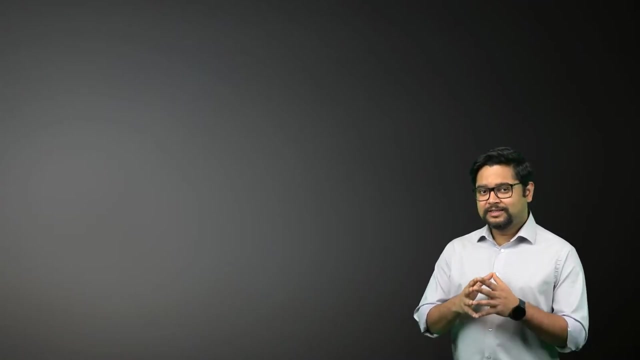 of this lesson. Natural convection occurs due to a buoyancy force that acts on a fluid having density gradients. These density gradients are usually due to temperature differences. In the case of natural convection, the flow velocities are generally smaller than those associated with the forced convection and therefore the corresponding convection heat transfer rates. 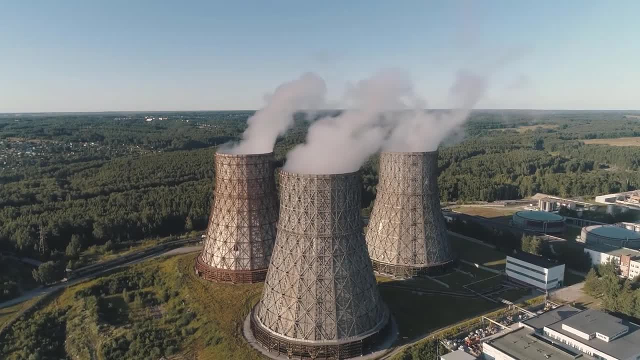 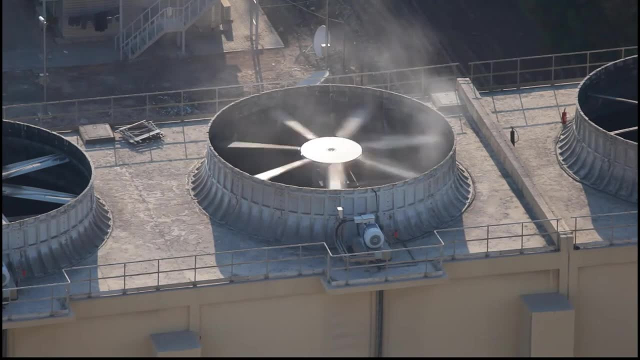 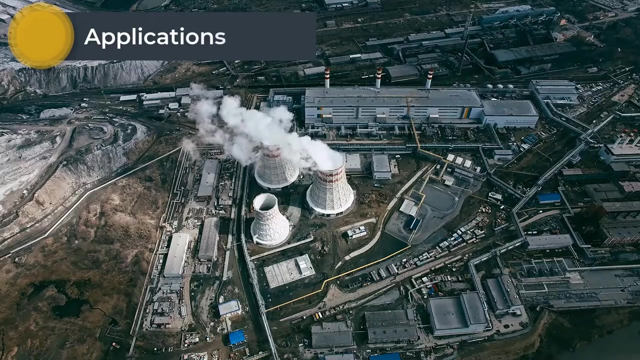 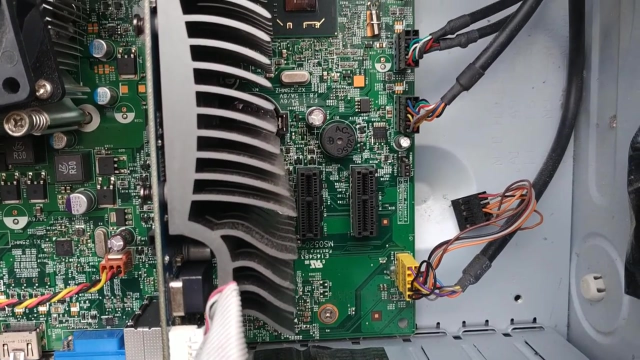 are also smaller. As a result, applications relying on natural convection are typically larger in size compared to their forced convection counterparts. Natural convection plays a very important role in many industrial applications, such as power generation, HVAC systems, electronics cooling. Moreover, it is the driving force 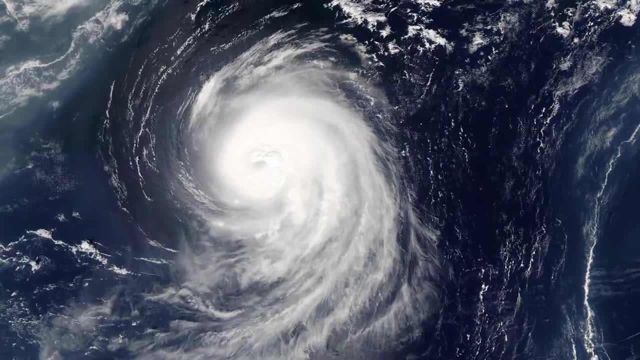 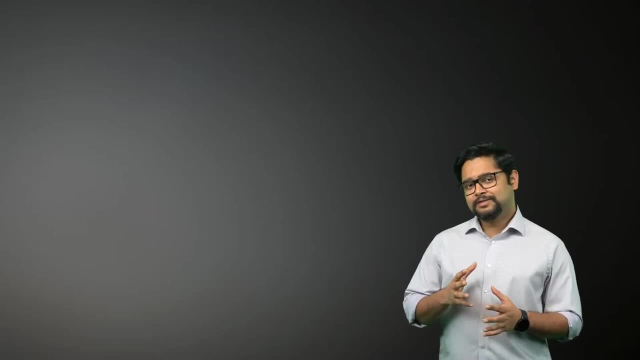 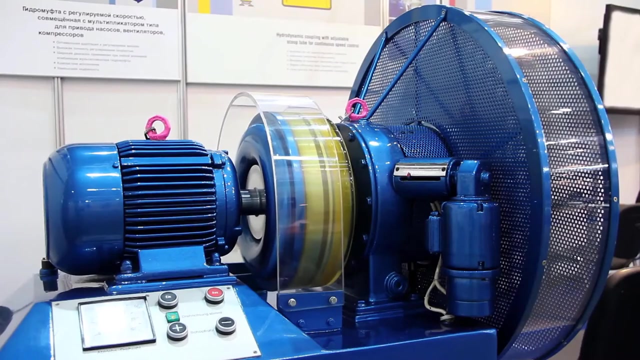 of many natural processes, such as ocean and atmospheric currents, The buoyancy-induced flow in a fluid is driven by an external body force when density gradients arise due to temperature differences. In most cases, this body force is gravitational. However, it can also be centrifugal force, for example in the case of rotating machinery, or it can 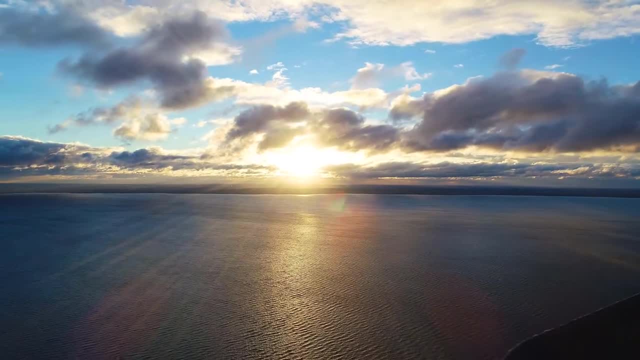 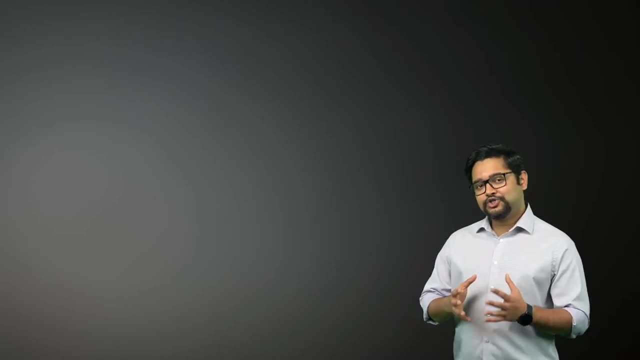 also be Coriolis force. as in the case of oceanic and atmospheric currents, Density of fluids depends on temperature, and it generally decreases with increasing temperature. This is because, as the temperature increases, the fluid expands and its volume increases. In this course, we will focus on natural convection, in which density gradient is due to a temperature. 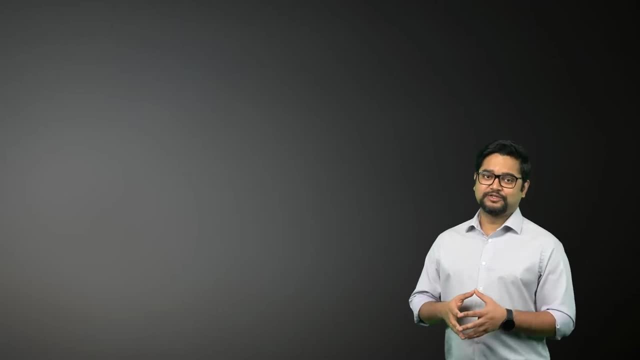 variation and the body force is gravitational. Now let's explore these natural convection currents in detail using the following example. Consider the conditions shown here. The fluid is enclosed by two large horizontal plates where the lower plate is at a higher temperature than the upper plate. As a result, the density decreases in the direction of 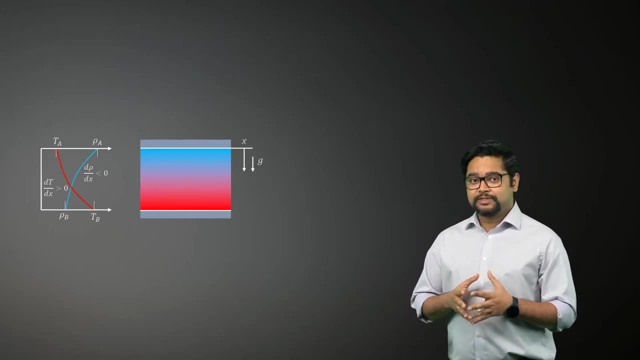 the gravitational force. If the temperature difference is such that the buoyancy forces can overcome the viscous forces, the fluid circulation would begin. The heavier fluid will descend, being warmed in the process, while the lighter fluid will rise and the heavier fluid will cool down as it moves. On the other hand, if the temperature of the 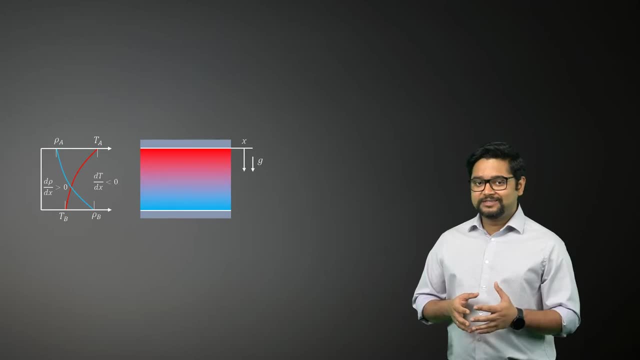 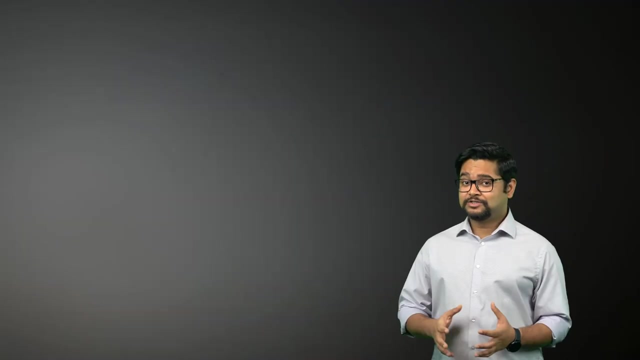 upper plate is higher, then the fluid density will not decrease in the direction of gravity and the flow pattern will not set up. In this case, heat will be transferred from the upper plate to the lower plate, but it will be via conduction and radiation. 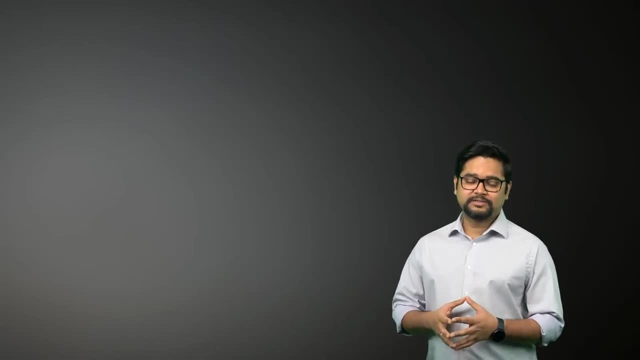 Natural convection can occur in many different types of settings. For example, we can have unbounded natural convection, in which the buoyant currents move in the absence of any bounding surface. Two common examples are plume formation over an immersed heated object and buoyant jet from a heated discharge in a cooler fluid. A plume is formed from the. 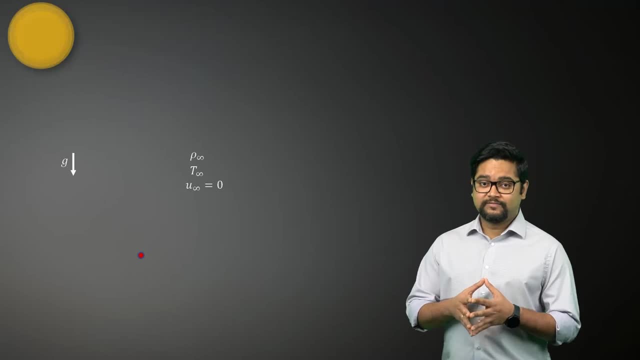 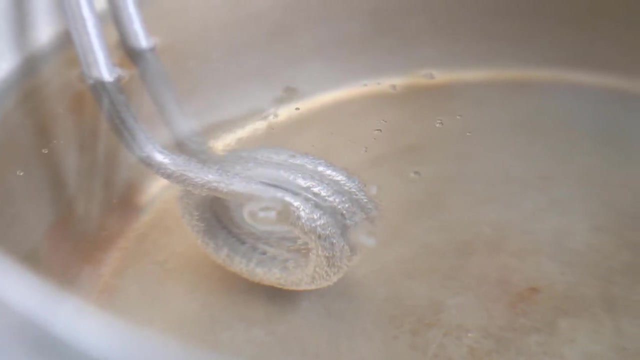 fluid rising from a heated object submerged in a quiescent fluid. The hot fluid rises due to the buoyancy forces and entrains more fluid from the quiescent region. The plume formed from a hot immersion water heater is a good example of this type of natural 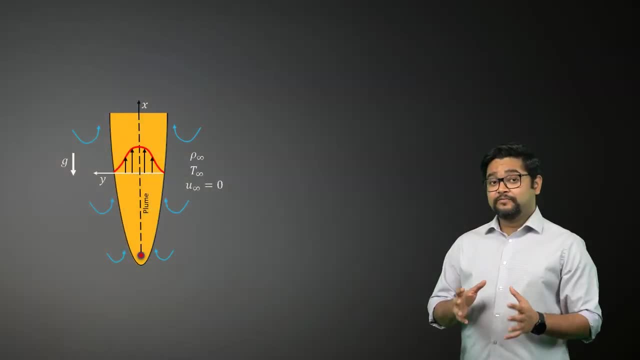 convection flow. The width of the plume increases with distance from the heated object. However, the plume itself eventually dissipates due to viscous effects and reduction in the buoyancy forces. Unlike plumes, buoyant jets have some initial velocity. as shown, They arise when a heated 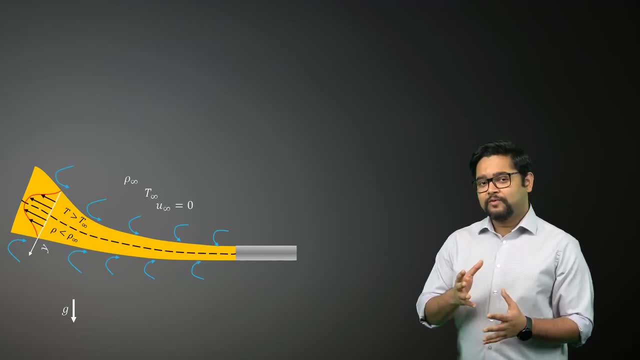 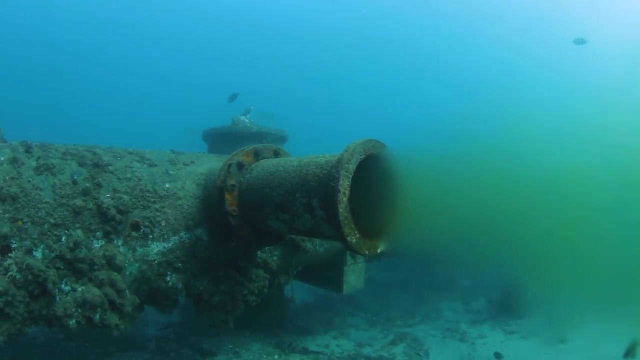 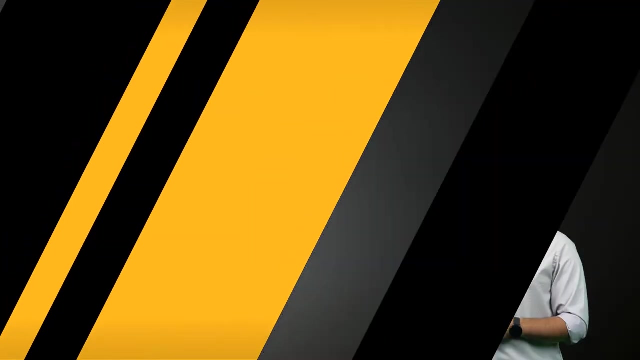 house is being discharged as a jet into a medium of lower temperature. Because of the buoyant forces, that jets gains a слب₮ ✧₺�. hi₃ Saw ✧₃, мы свои. And other natural convection flows arise when the soil with broontonieni are haveoyu. 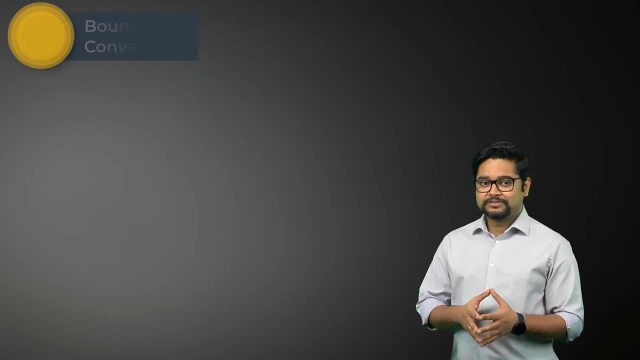 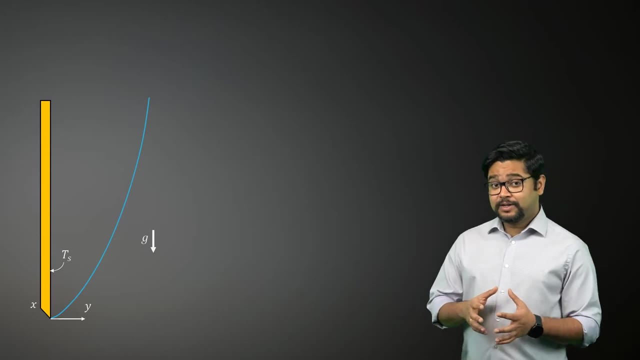 near from the iht órоз Enlightened 시 carved 既 ڡ₁ает surface. a canonical example of such flows is the boundary layer development on a heated vertical plate. this plate is fully immersed in an ambient medium having a lower free stream temperature. 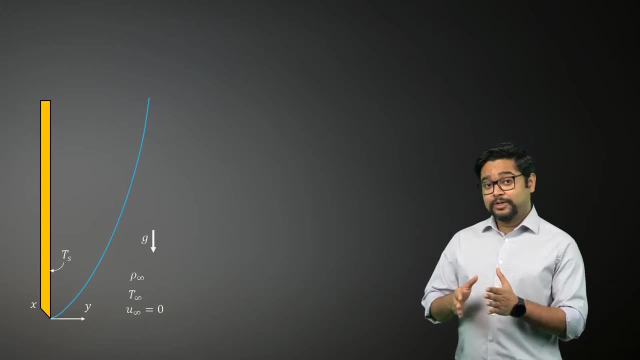 than the plate. as a result, the fluid close to the plate is former compared to the fluid that is further away from the plate. this makes the fluid close to the plate less dense and the buoyancy forces induce a free convection boundary layer in which the heated fluid rises vertically. 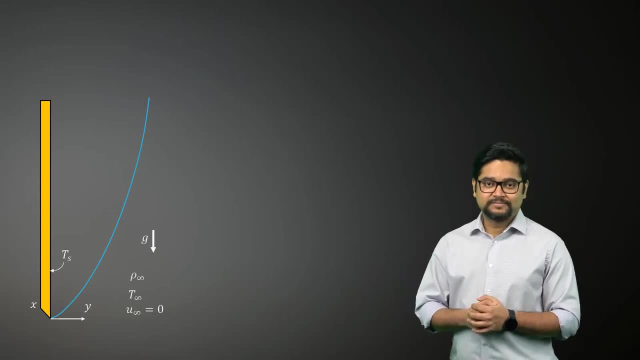 and in the process, entrains more fluid from the ambient region. the resulting boundary layer is different from the one we get in the case of forced convection. this is because the velocity is zero as y approaches infinity and as well as when the y is equal to zero close to the wall, a natural convection boundary layer will also develop. 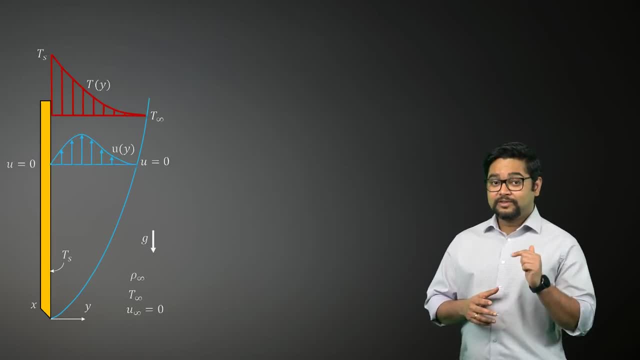 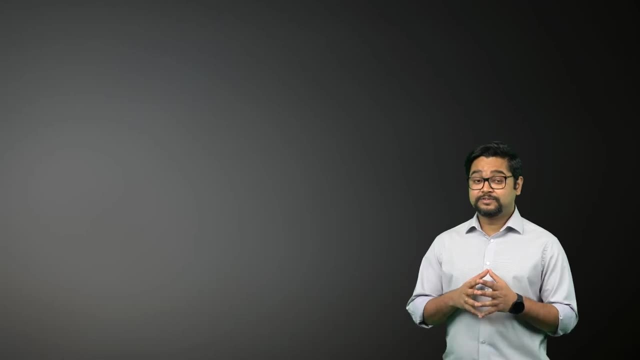 if the plate is immersed in an ambient medium. and if the plate is immersed in an ambient medium, the flow towards the wave will be split into two and that means it bzw will be of other holiness exhaust's fluid. in a hotter fluid, however, the fluid motion 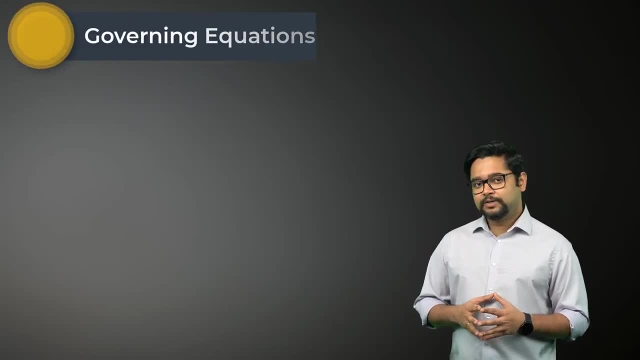 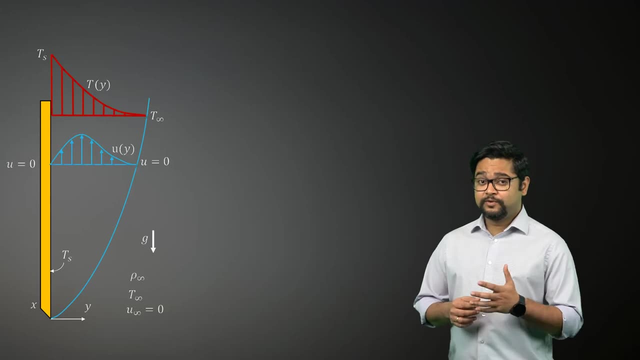 in this case, will be downwards, as shown here. now that we have some understanding of natural convection, let's quickly look at its governing equations. consider the lamina boundary layer flow shown here. we assume the flow to be two-dimensional, steady, with constant property conditions, and we assume that the boundary layer approximations are valid. 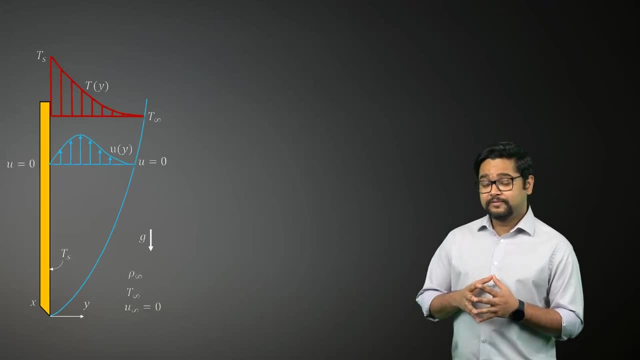 as soon as chega happens on the gذ, the nav율35a will begin to move downward. the landscape of the volume TurHa will weigh half to make a new tan fo přòd level ane, With gravity acting in the negative x direction. the x-momentum equation can be written as: